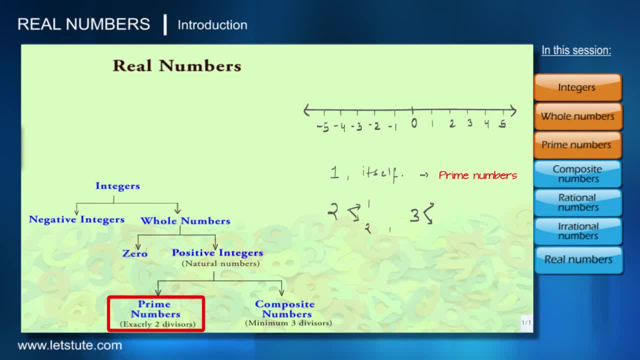 Similarly, 3 has two devices, that is 1 and the number itself. 5, 5 has exactly two devices, that is 1 and the number itself, and so on. So 2,, 3,, 5, they are all prime numbers. 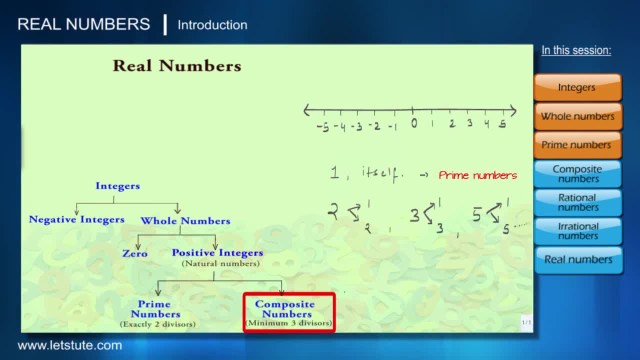 And composite numbers are the numbers which has at least three devices or more than that. For example, 4 has three devices: 1,, 2, and 4, that means 4 can be divided by 1,, 2, and 4.. 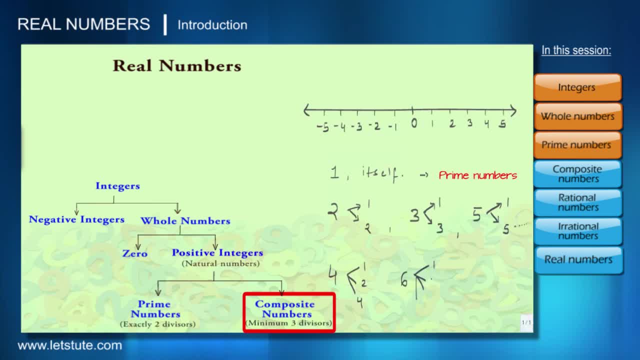 Similarly, 6, 6 has four devices, that is, 1,, 2,, 3, and the number 6 itself. So they are all composite numbers. But we also know that the number 1 is the only number which has only one divisor. 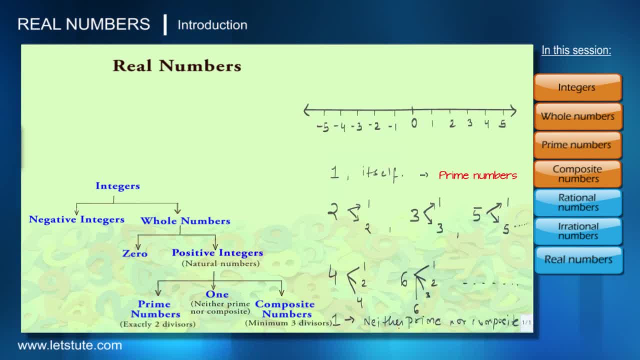 So 1 is neither prime nor composite. Now, on the other hand, we have two devices. Now, on the other hand, we have two devices, that is, 1 and the number itself, and so on. On this number line, in between these integers, there are many more numbers that are present in the form of fractions, or we can say, decimals. 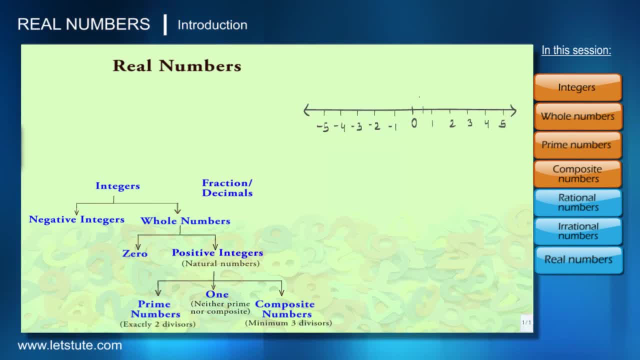 For example, in between 0 and 1, there is a number 0.5, or in terms of fraction, I can write 0.5 as 1 by 2.. Similarly, in between minus 2 and minus 3, there is a number minus 5 by 2, or in terms of decimal, I can say minus 2.5. 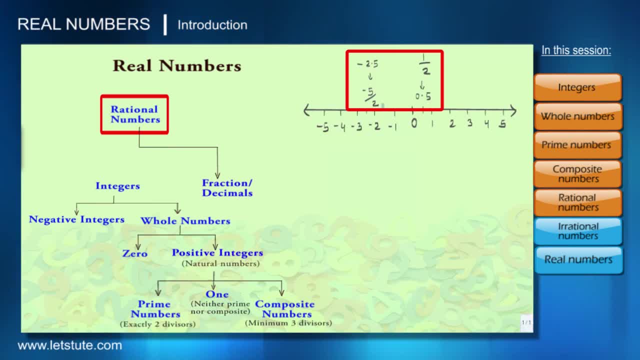 Similarly, in between minus 2 and minus 3, there is a number minus 5 by 2, or in terms of decimal I can say minus 2.5.. In this way the fractions are called as rational numbers. The word rational comes from the word ratio. 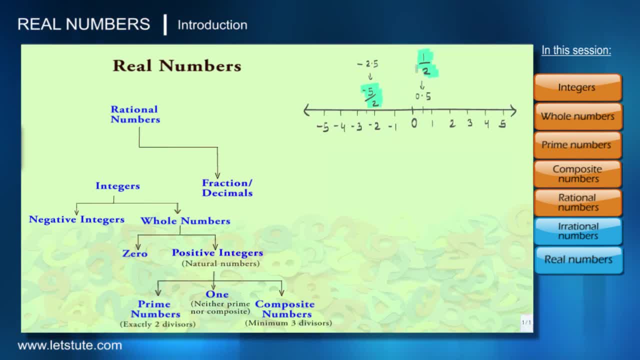 As we can see here, 1 by 2 and minus 5 by 2 are nothing but the ratio of two integers, So they are called as rational numbers, And note that every integer is also a rational number, As we can write the integer 0 as 0 by 1, 1 as 1 by 1, 2 as 2 by 1, and so on. 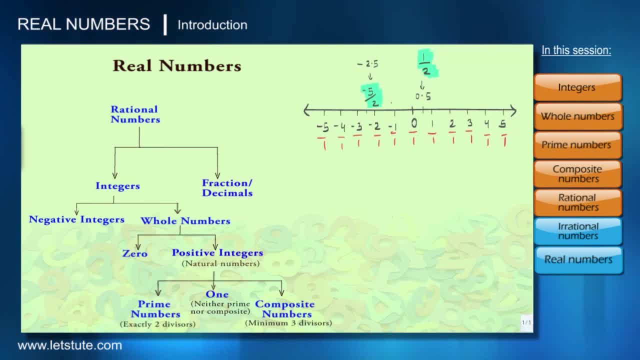 And we also know that rational numbers can be written in the decimal form form, and this decimal form can either be terminating or non-terminating. for example, we know that 3 by 2 is a rational number and decimal form of 3 by 2 is nothing but 1.5. so here 1.5 is.